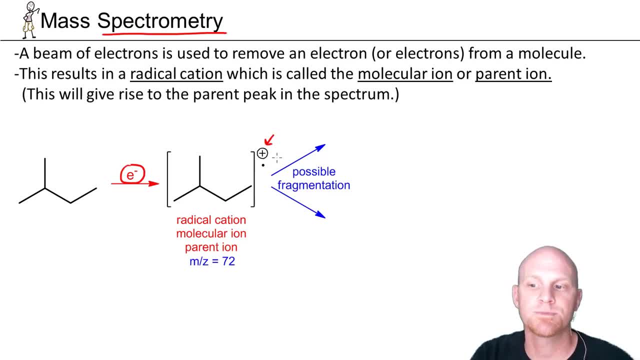 electron out of a molecule. That's going to leave the molecule both with a positive charge but also with an unpaired electron somewhere. So having a positive charge, we'll call it a cation, Having an unpaired electron, we'll call it a radical. Overall that makes it a radical. 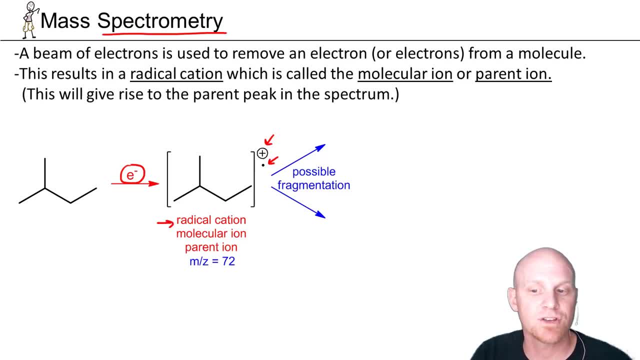 cation, An electron weighs just some small fraction of an AMU, So this really hasn't lost much for mass. So your radical cation here has the same molecular weight as your original compound. So we call it the molecular ion. So we'll also sometimes call it the parent ion, as we'll see. 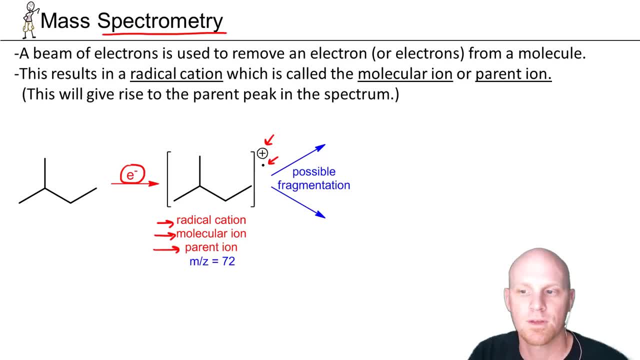 in a little bit, that it's going to give way to the parent peak. So when we hit a molecule and knock an electron out here with this beam of electrons, we're going to make it unstable as well, And it might actually break into fragments, as we'll see. 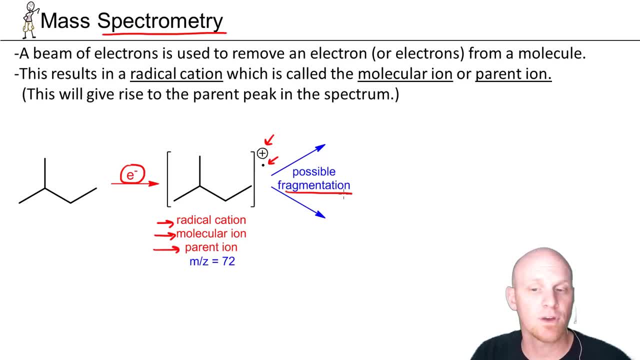 But you're not just doing this with one molecule, You're doing it with a zillion molecules, So some will stay together. potentially, Some will break into this fragment, Some will break into that And we'll find out that the more stable the fragments it can break up into, the more those 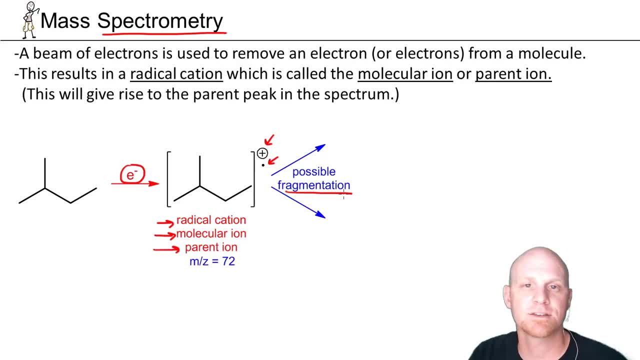 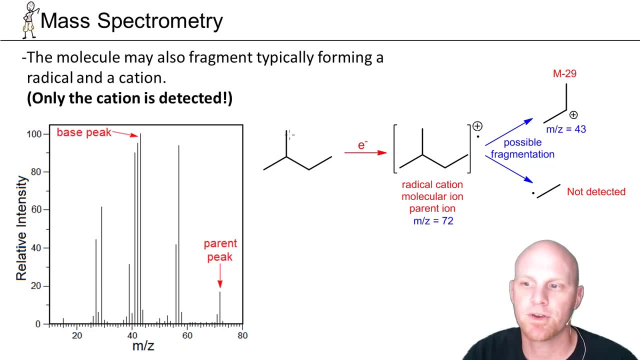 fragments will form, It'll give a higher intensity peak on the mass spectrum. So let's take a look at some of these possible fragmentation patterns. If we look at the original molecule here, we often classify carbons based on how many other carbons they're bonded to. So this would be considered a primary carbon, being only bonded. 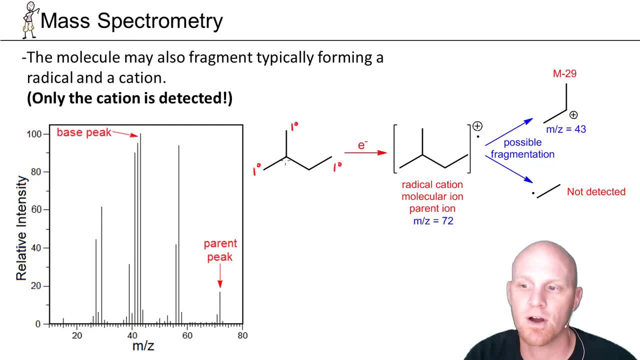 directly to one other carbon. This also is a primary carbon, and this is a primary carbon, But this one being bonded to two carbons would be considered secondary, and this carbon bonded to three carbons would be considered tertiary. We'll find out that our alkanes often fragment. 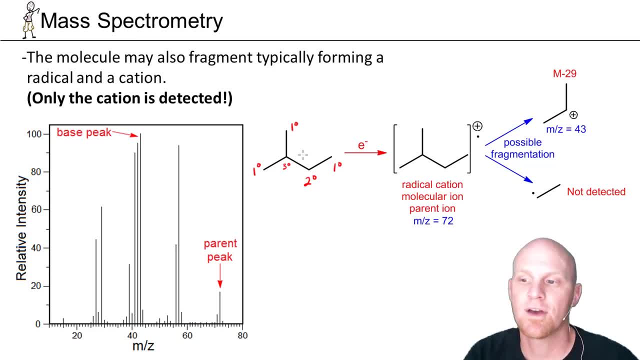 in between the two most substituted carbons. if there's two most substituted carbons, And that's going to be the case here- and that would be fragmenting right here between the tertiary and secondary carbon. So let's just envision for a moment. 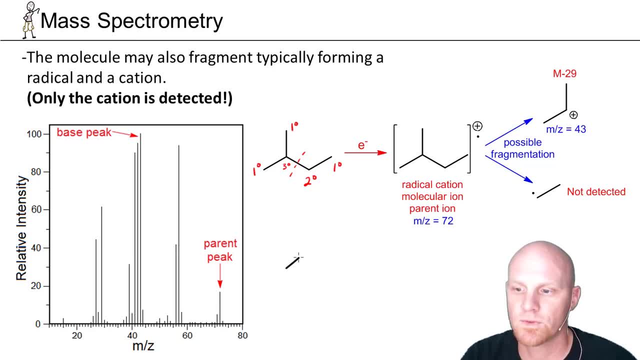 that in this molecule. so we're going to redraw it and we're going to draw the fact that that bond is made up of two electrons. Well, we're going to knock one of those electrons clean out, so he's just gone. 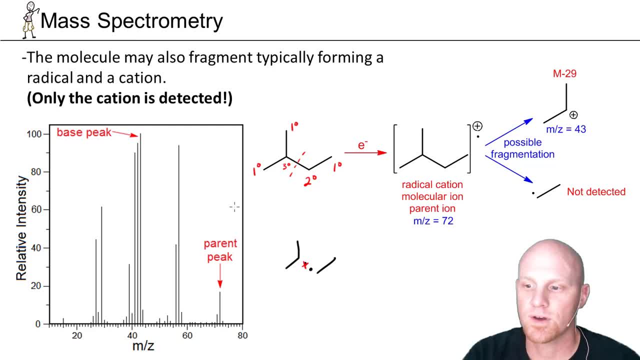 So I'll cross him out there, And so what you're left with is a couple of different fragments here, So and one's going to be a carbocation. So typically we make, the more substituted side is more probably going to be the carbocation. 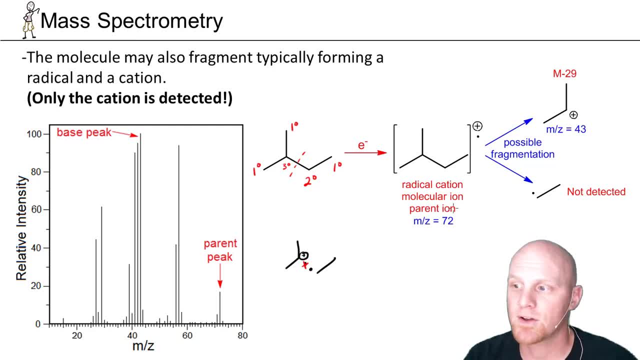 being more stable that way, and the less substituted side will end up being the radical. So that's how we get these two fragments at the end of the molecule. That's what I've got depicted So off to the right here. Cool, So it turns out: more substituted carbocations and more substituted radicals are more stable. 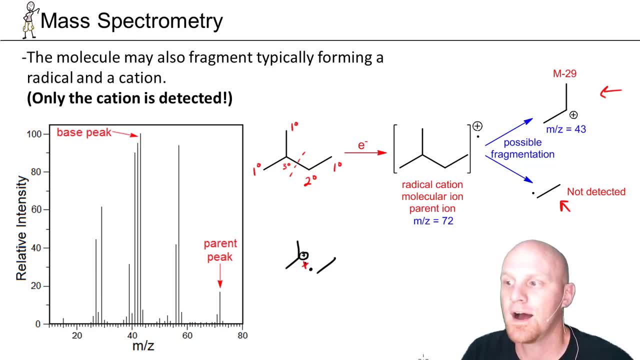 and that's why we broke between the most substituted carbons with our alkane. here, Turns out, the cation is what we'll actually detect in our signal here, And we might call this an M minus 29 signal here, because we're losing this ethyl group as it broke. 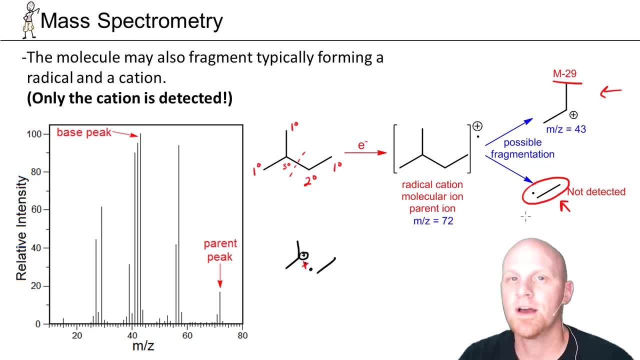 And an ethyl group weighs 29,. but we're not going to see it. It turns out you've got to be charged to be visible in mass spectrometry. We're actually going to accelerate charged particles toward the detector. We do that with a magnetic field. We can deflect them into the detector. 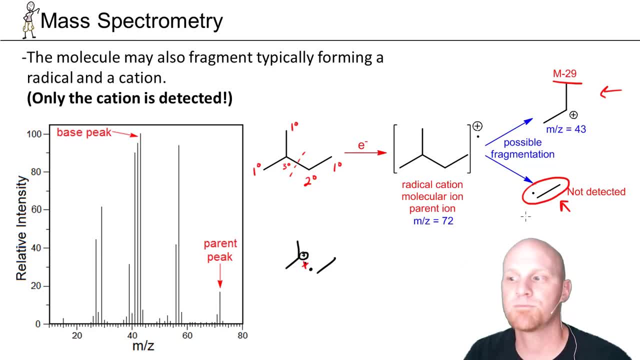 but a magnetic field will only operate on a moving charged particle. So this radical down here that is not charged will not be detected at all. So only positively charged fragments, it turns out, are going to see in our mass spectrum here. One other thing to note: if you look, everything's kind of listed in M over Z, M over Z. 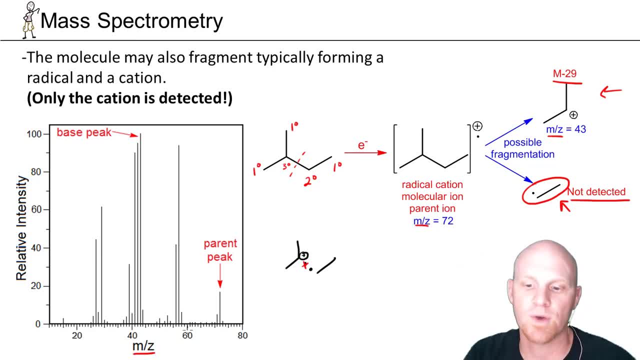 and even the x-axis on the spectrum. M over Z. That's the mass to charge ratio. So M for mass, Z for charge. The peaks we're going to look at are largely only going to have a plus one charge. so mass over plus one equates to mass. 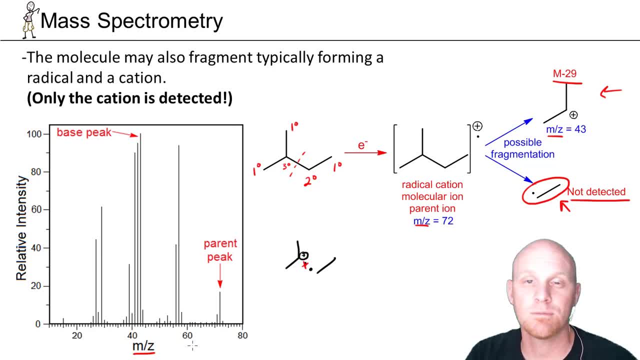 So keep in mind, we'll be treating this x-axis largely as mass. but keep in mind you should know it is mass to charge ratio formally. So if we look here we found out that our molecular ion here had an M over Z of 72,. 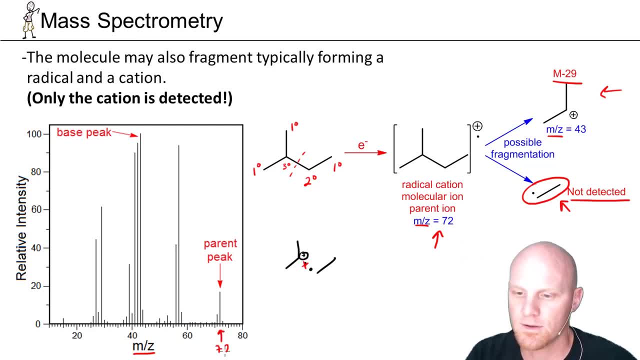 and we can see that right here on our mass spectrum. You look at another thing called our base peak and the base peak is just the overall tallest peak on the spectrum and it's going to be given a relative intensity of 100% and everything else is kind of relative to that base peak. 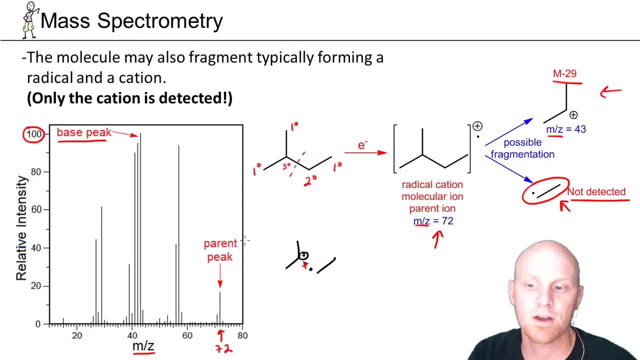 Sometimes your base peak and your parent peak are two different peaks, but you should remember that your parent peak is for your molecular ion. it gives you your molecular weight. Your base peak is just the overall tallest peak on the spectrum. So notice also our M minus 29 peak that we talked about over here. 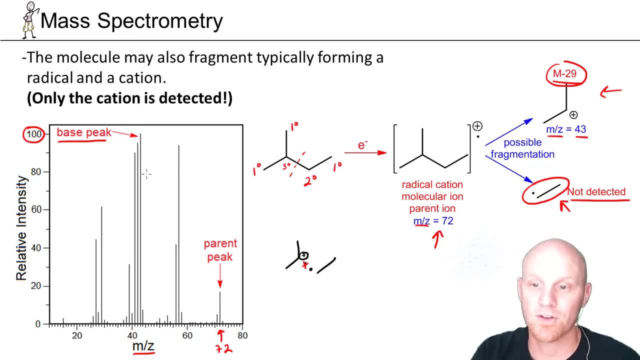 So it itself has an M over Z of 43, and, if you notice, our base peak is corresponding to that 43. So our base peak actually is the secondary carbocation that we've labeled the M minus 29 peak, the loss of an ethyl group. 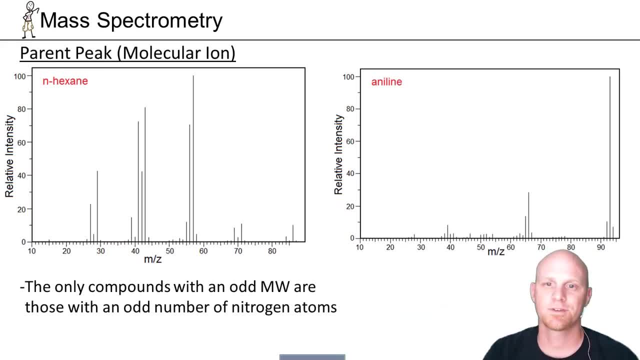 So if you're interpreting some mass spectra, first thing I recommend you do is actually find your parent peak. So again, your parent peak might- I should say your parent- ion might fragment into smaller pieces, but it can't form any larger pieces than that. 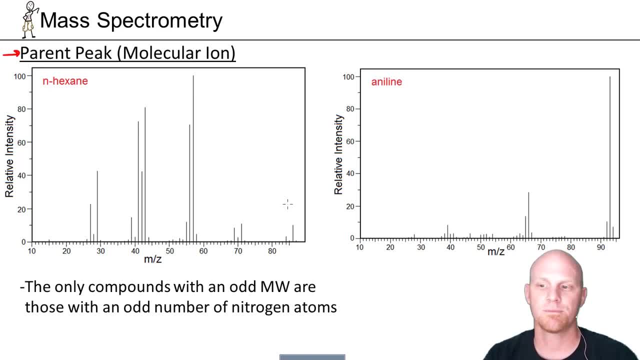 So if you go to the far right of your spectrum here, so usually the peaks are going to appear in clusters due to some isotope effects and stuff like this. but look for the tall peak in that cluster and that's your molecular ion. 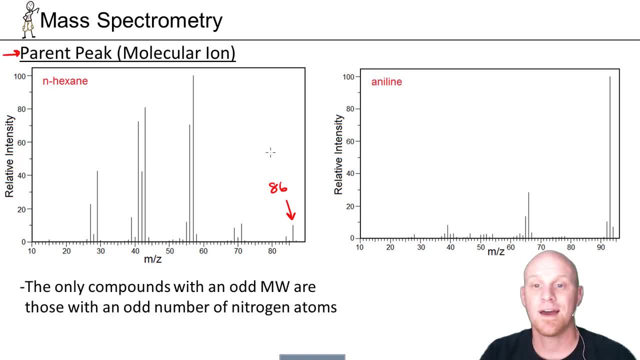 And so for this compound we see it's at 86, and indeed hexane has a molecular weight of 86.. So for the compound on the right here, we'll go to this cluster of peaks, all the way down here and the tall peak in that cluster. 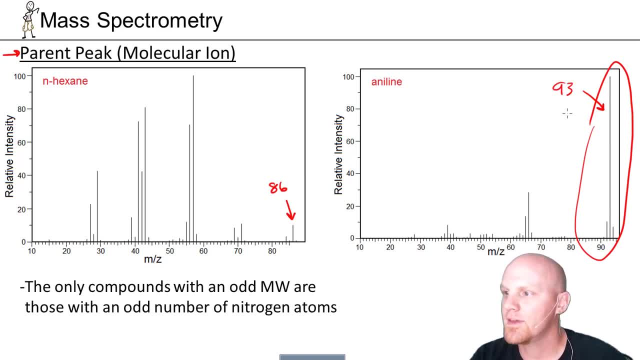 if we look, weighs 93.. And that's a number that's going to stick out at us Anytime you see an odd-numbered molecular weight for your molecular ion, specifically, that tells you you've got nitrogen in your compound and specifically, 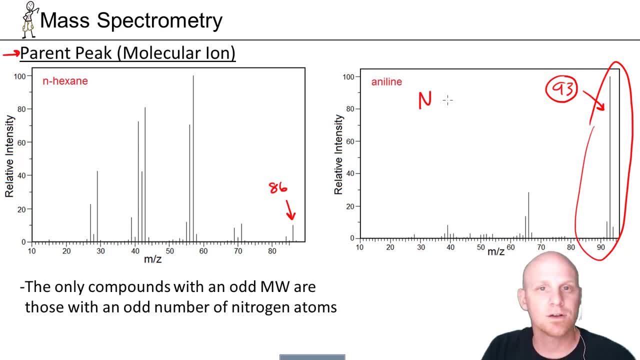 it tells you you have an odd number of nitrogens, in this case one nitrogen. Technically, if you have two nitrogens, you'll come back out with an odd molecular weight, I'm sorry, an even molecular weight. 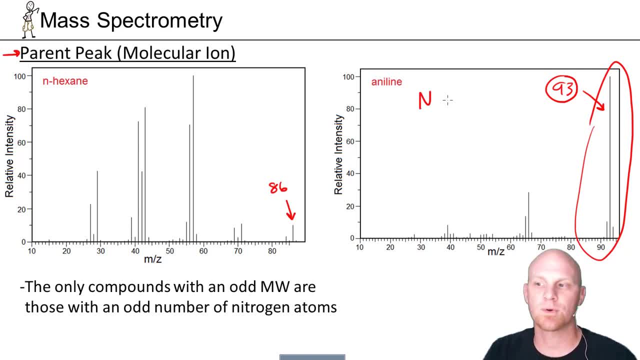 but with three nitrogens you go back to being odd. Well, most of the time you're really going to be dealing with one nitrogen or none. Every once in a blue moon, some professor will slip in a couple there. two nitrogens. 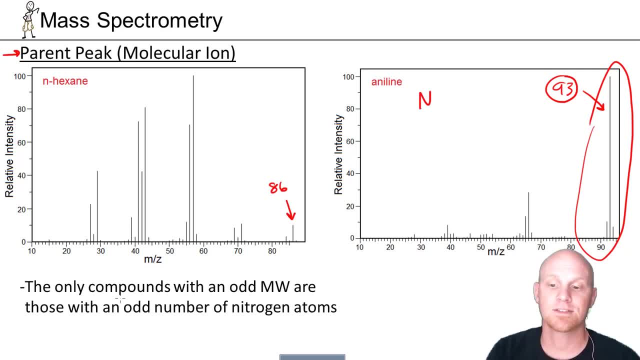 and get back to an even molecular weight. but it's not common, And the key here is that the only way you come out with an odd molecular weight is if you have an odd number of nitrogen atoms. It's just kind of a pure coincidence here. 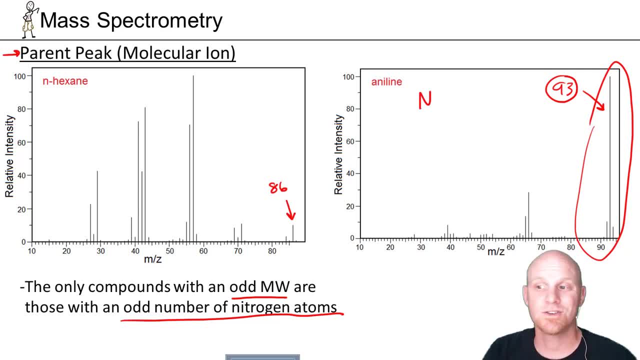 In mass spectrometry of organic compounds. unless you have nitrogen, you can never get an odd molecular weight. It's a beautiful thing. So when you get that odd molecular weight right off the bat, you know you've got nitrogen in your compound. 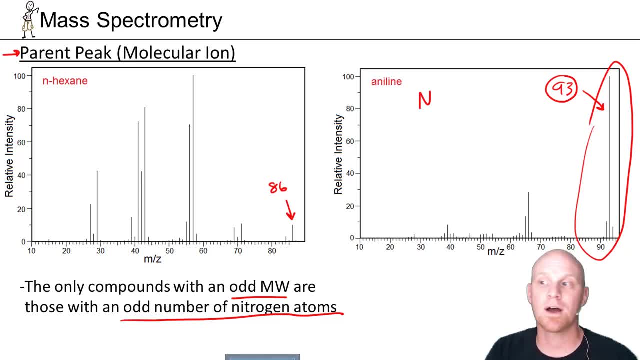 So again, find that parent peak. at the very least get your molecular weight of a compound, and if it's an odd number, bonus. you know you have nitrogen in your compound as well. 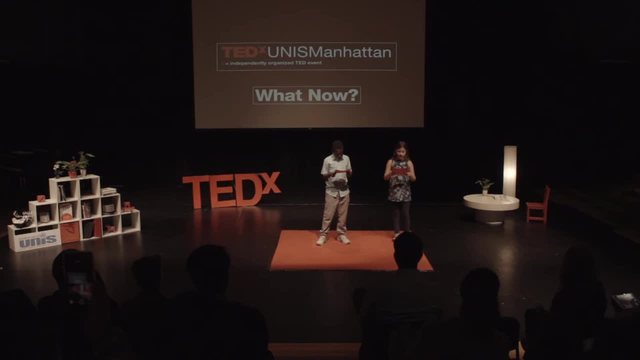 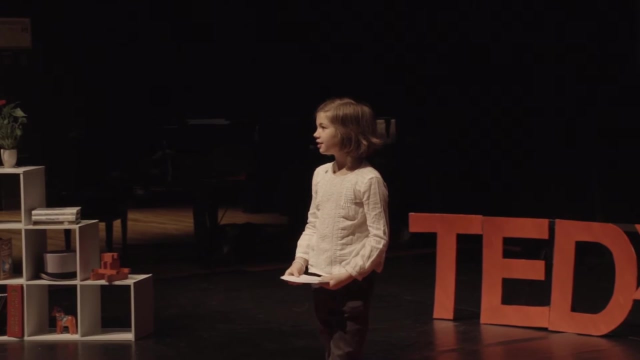 To open our morning session, I invite our first speaker, Talam, who is an M1 student. She will be sharing her idea on how sports can have a very positive impact on the lives of children. Welcome, Talam. Hey everyone, Thanks for inviting me here today to be a TEDx Talk speaker.